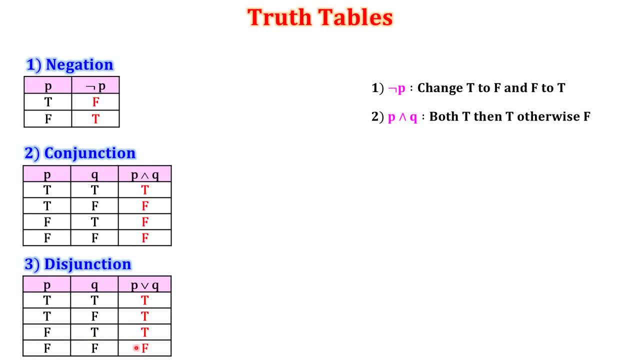 both are false, then the answer is false, otherwise true. so remember for P, R, Q: if both are false, then answer is false, otherwise true. next fourth, one conditional statement. consider two statements: P, Q, that is TT, TF, FT, FF. the conditional is denoted like this: P, then 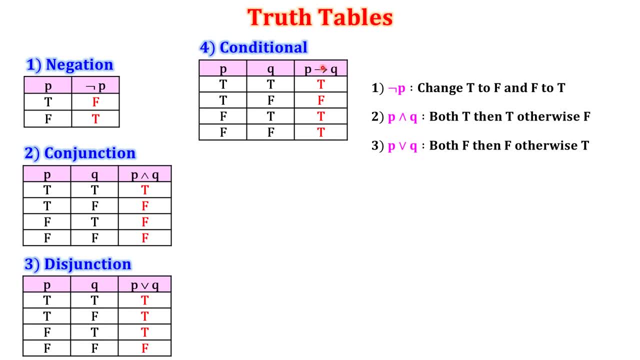 Q single arrow mark. we say that P then Q, Q. here the first statement true, second statement: false, then the answer is false, otherwise true. here the first statement is P, so P is true. second statement: Q is false, then we get the answer false, otherwise true. so P then Q. we can. 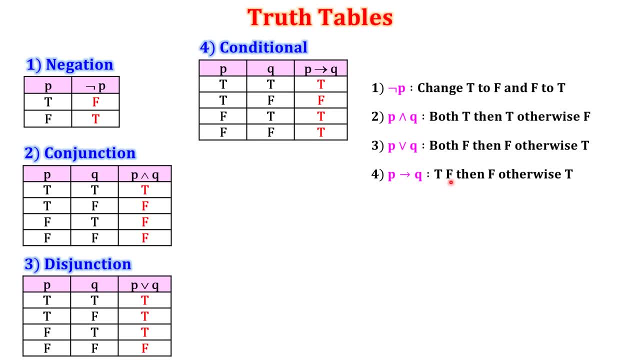 remember like this easily: T, F, then the answer is F, that is first true, second: false. then the answer is false, otherwise true. next, fifth biconditional: here also we have two statements, P, Q and four possibilities: TT, TF, FT, FF. the biconditional is denoted. 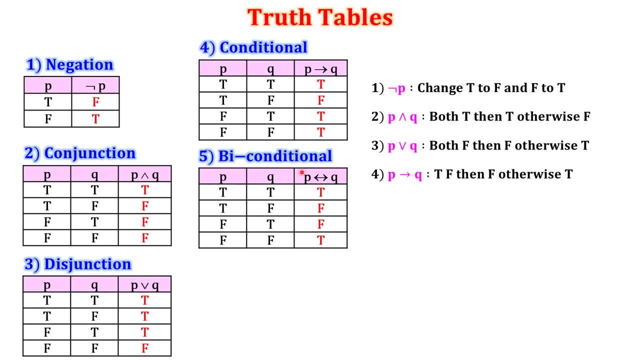 like this: P, if and only if, Q. so double side arrow mark. we say that if and only if. Here the condition is: if both are same, then the answer is true, Otherwise false. Both are same means: see the first row: true, true. 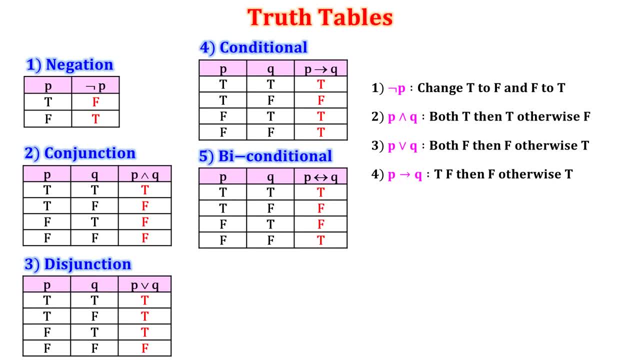 then the answer is true. See the last row f, f same, then the answer is true, Otherwise false. So the biconditional p: if and only if q. we can remember like this: if both. 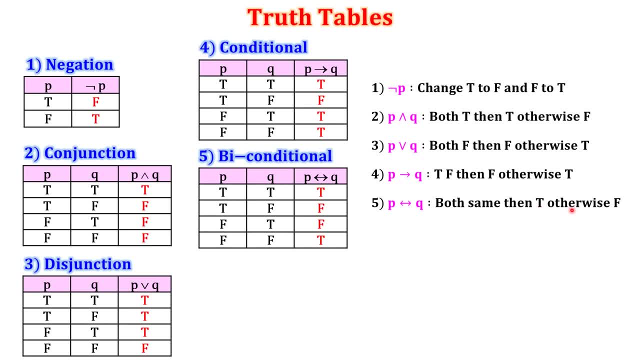 are same, then the answer is true, Otherwise false. And sixth: exclusive or. Here also we have two statements, p, q, and four possibilities: t, t, tf, ft, ff. The exclusive or is denoted like this: p x, r, q. Here the condition is if both are same. 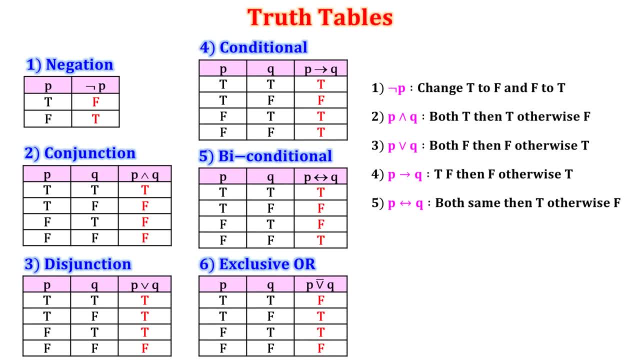 then the answer is false, Otherwise true. See the first row t, t same. last row f, f same. So for that we have to put the answer: false, Otherwise true. So remember p, x, r, q. The condition is: if both are same, then false, Otherwise true. So these: 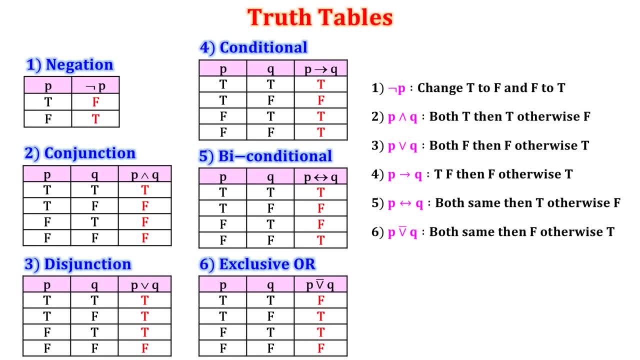 six are the logical connectives. we use it in problems And in the truth tables. false is the first one. Finally, if we get all the answers true, then we say that it's a tautology In the truth table. if the final answers are false, then we say that it's a contradiction. 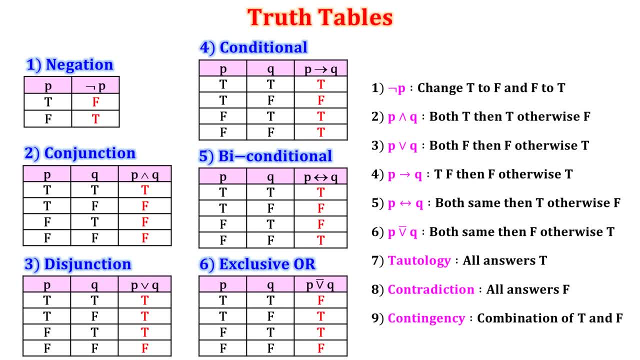 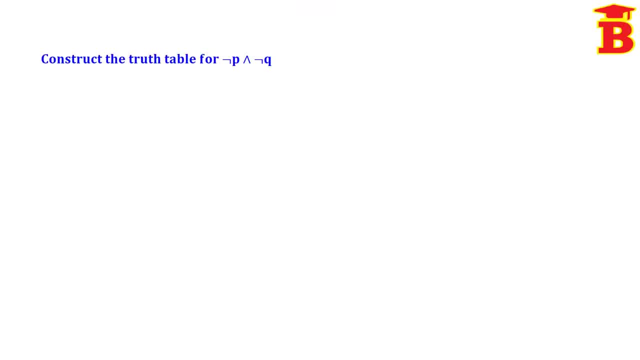 If we have both mixed true and false, then we say that it is a contingency. Now let us see the problems. Construct the truth table for not p and not q. Now we have to draw the truth table and we have to use the conditions Instead of remembering all the tables. it. 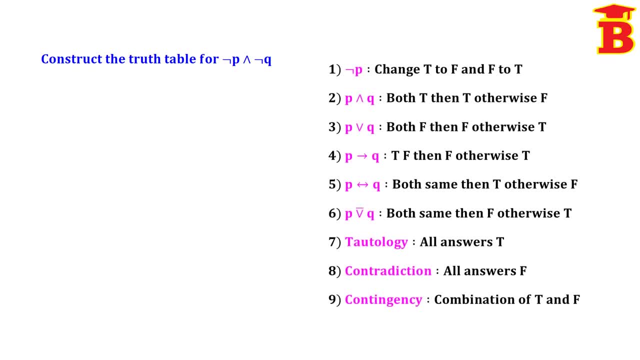 is very easy if we remember these conditions. Now we have to take two statements: p, q. We know that there are four possibilities: tt, tf, ft, ft and ftx. There are four possibilities: F, T, F, F. Here see the question and draw the table In the question. first, we have not P. 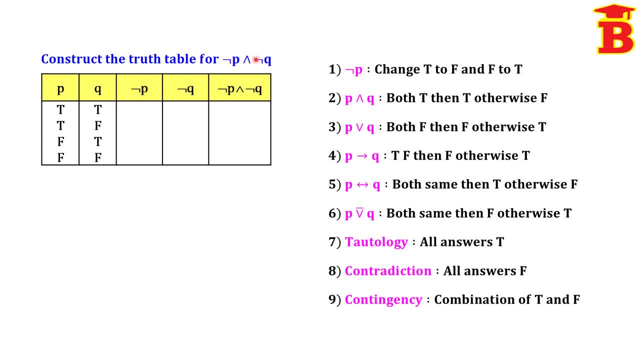 So in the table also we have to take not P. In the question next we have not Q, So in the table also. next, take not Q and final column. see the question and take and write it: not P and not Q. Now we have to find not P. Not means change T to F and F to T. So see the. 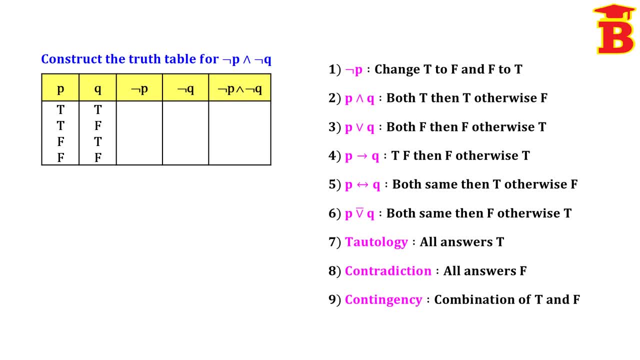 statement: P just change T to F and F to T. So first one, T, we have to change it as F. Second, T, change it to F. Third, F. Fourth, F- change it to T. Fourth also F, change it to T. So this is negation, not P. Similarly, 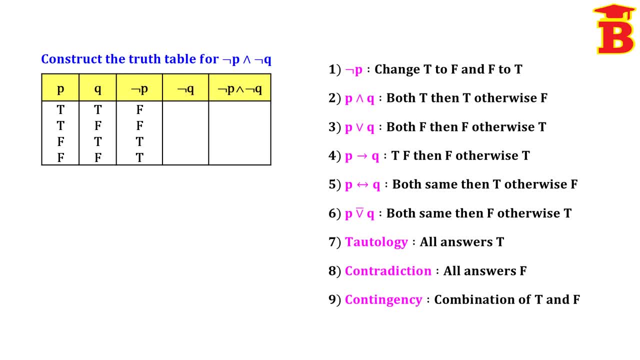 next column, not Q. We have Q Here. also we have to use negation, not Q. So see the statement. Q change T to F and F to T. So first one T change it to F and F to T, So see the statement. 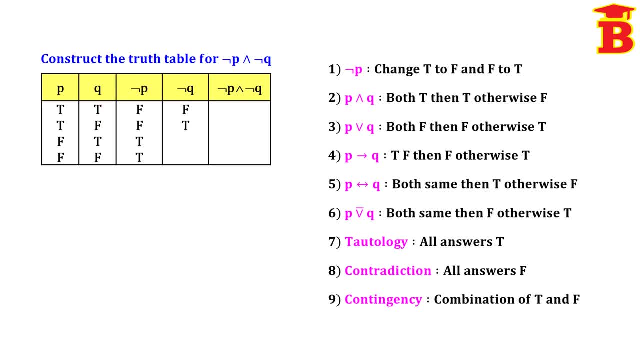 to F. Second F: change it to T. Third T: change it to F. Fourth F: change it to T. And now, finally, not P and not Q, For these two we have to take, and P and Q means both- true. 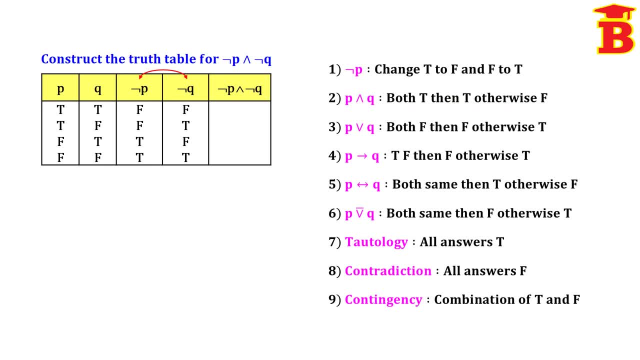 then answer true, Otherwise false. So to take: and for these two we can use the condition very easily like this: If both are true, then the answer is true. Check in these statements whether we have both true. Only in the final row we have both true. So for that we have. 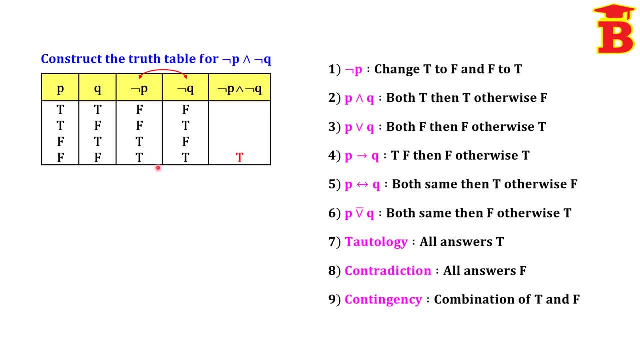 to write true. So both true means answer true, Otherwise false. So for all the remaining we can write false F. So this is the final answer: F, F, F, T. Similarly, next is some construct the truth table for negation of P and not Q. So here also there are two. 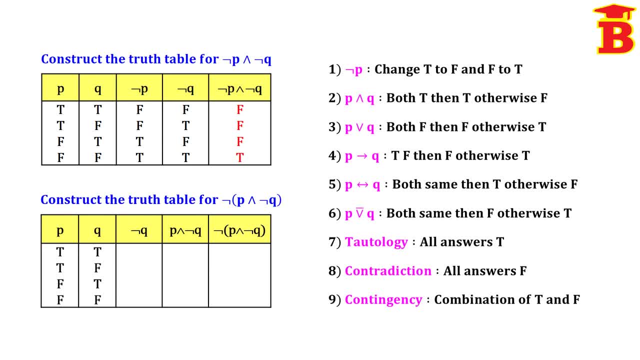 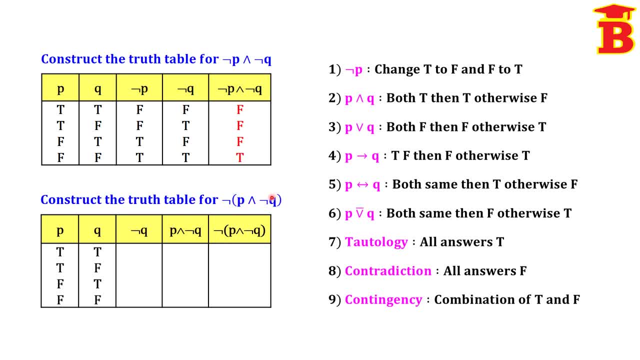 we have not Q. So in the table also write not Q and then take this bracket P and not Q and finally negation of P and not Q. Here first one, not Q. We have the statement Q Not Q means just change T to F and F to T. So first this T, change it to F. Second, 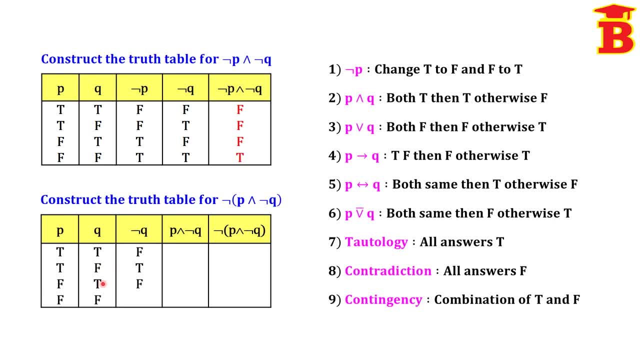 F, change it to T. Third T, change it to F. Fourth F, change it to T. Next P and not Q. So these two we have to connect using and, And note that and means both true, then true, Otherwise false. So in these two columns: 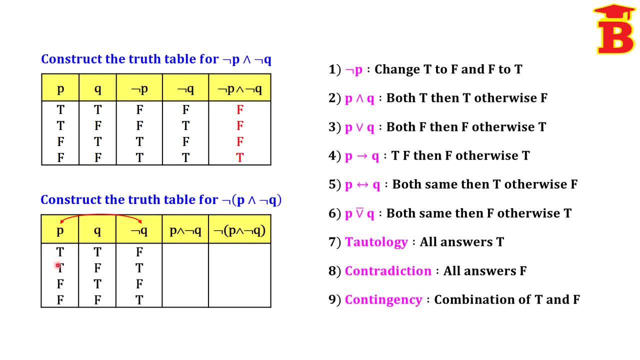 check whether we have both true. Only in the second row we have both true. So for that the answer is true, Otherwise false. So all the remaining false. We can write F And finally, not bracket, P and not Q. So this: we have to change T to F and F to T. So here F, change it to. 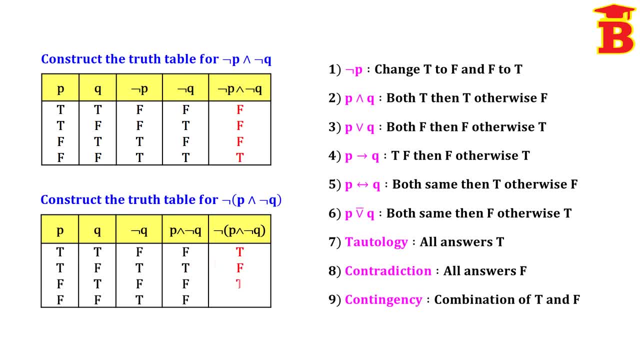 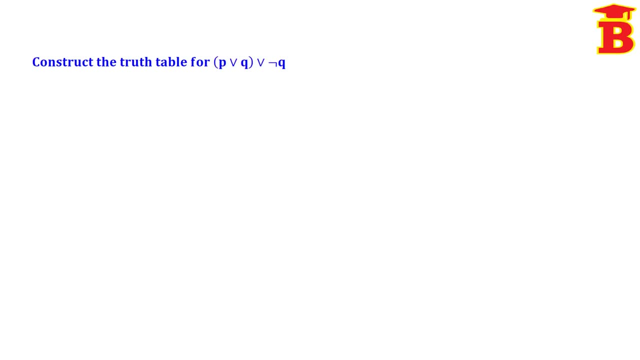 T, Next T change it to F, And then F change it to T And finally F change it to T. So this is the final answer: T, F, T, T. Similarly, next, construct the truth table for P, R, Q, R, not Q. So remember these conditions. 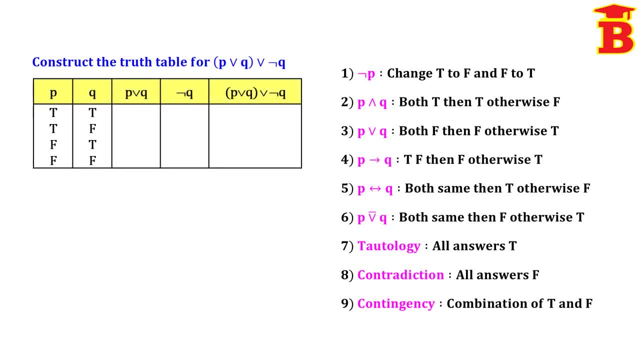 we can draw the truth table very easily: P, Q, two statements. So there are four possibilities: T, T, T, F, F, T F F. See the question and take the table. First bracket, P, R, Q. Next, not. 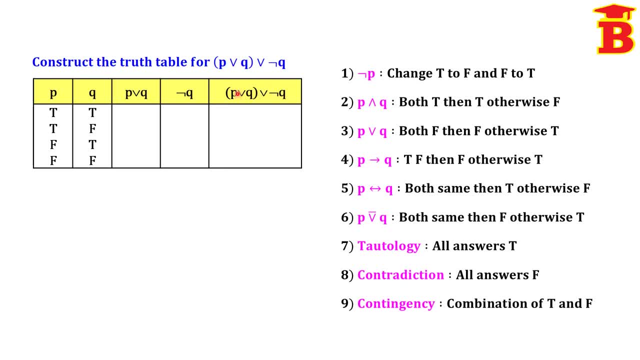 Q And finally question P R Q R, not Q P R Q. That means both false, then answer false, Otherwise true. So check whether we have both false. Only in the last row we have. 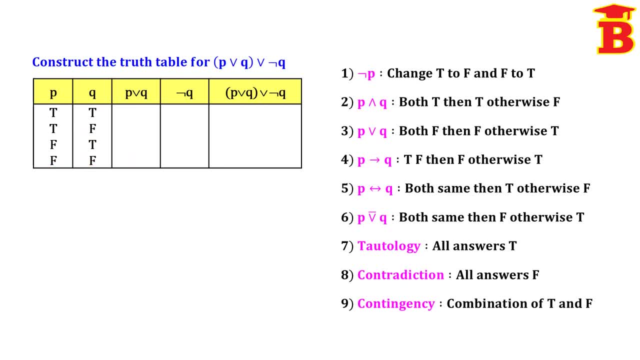 both false. Further, the answer is false Otherwise two, So all other answers true. Next column: not Q, So see the statement: Q change T to F, F to T, So T to F. Second, 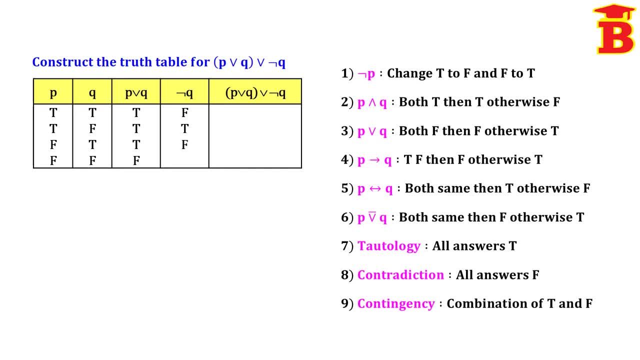 F to T, Third T to F, Fourth F to T. Now, In summary, if we take both statements, coming to master, a scheut class entry this from whatever row, and we already know that the proof of science for that is an 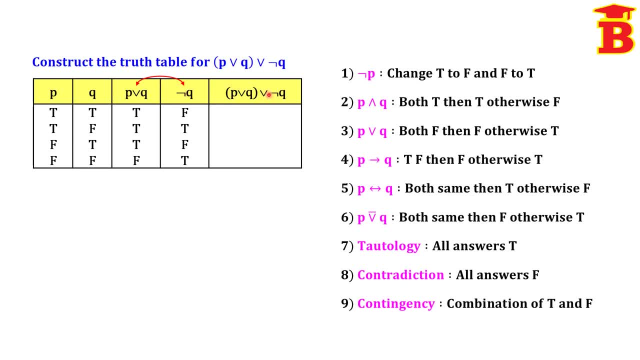 thon is the paisen brushing that? the proof of science for that is F Selection correction is immediately three weeks. it is good If there are four of us. it is good if you like it. The have to connect using R again. for R we have the condition: if both false, then 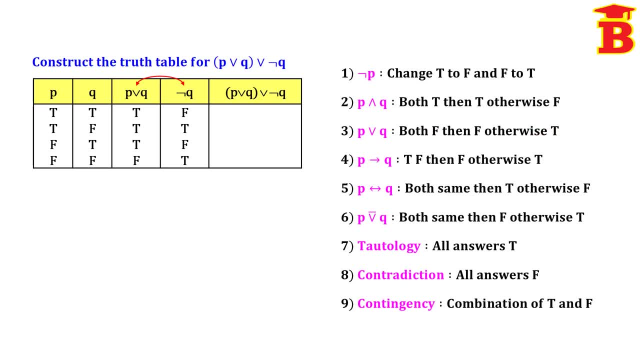 answer false, otherwise true. so check in these two columns whether we have both false. we don't have both false, that means all the answers are true. so the final answer: T T T T. next one: construct the truth table for P X R, Q and P X R. 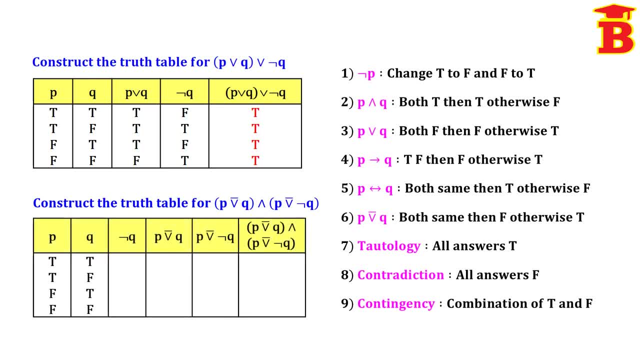 not Q. we take P Q, two statements and four possibilities: T, T, T, F, F, T F F. see the question and take the table. so take not Q and then first bracket P XR, Q and then second bracket P XR, not Q and finally take this question first, not. 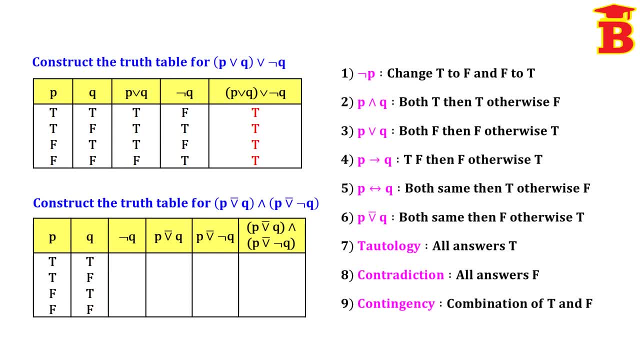 Q means we have the statement Q, just change T to F and F to T, next P XR Q. P XR Q means: if both false, then answer true. so check in these two columns whether we both same, then answer false, otherwise true. so check these two both same means. 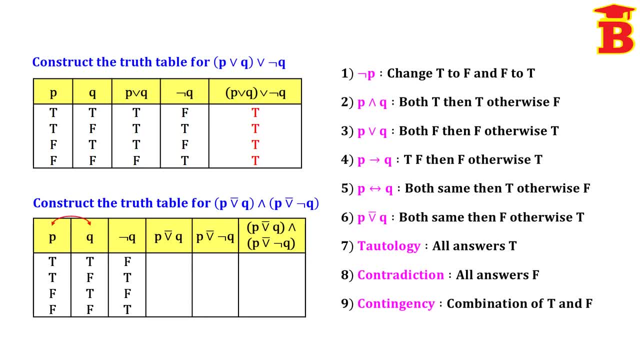 first row and last row. for that we have to write F, first row, last row: we have same, so for that we have to put F, otherwise true. so other two answers true: T, rule a: F, as we have nothing left. next step: P, X or not, Q. so for these two we have to. 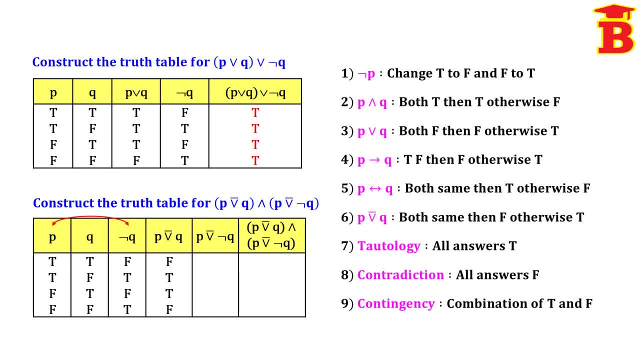 get X R. so check in these two columns whether we have same second row and the third row same. for that we have to write F, others true, so other two. and Sir T. final question answer says positive. so we have repeated answer negative. so the final statement: M, X. start with M position twice: T, Xaminz, D. all these answers are right. answer: or we заб abra IP available, D. next step: P, XR, 0, q. so for these two we have to be X, our. so checking these two columns whether we have same. so second row and third row 됩니다e. for that we have to write F, others true, so other two. answer D. finally, 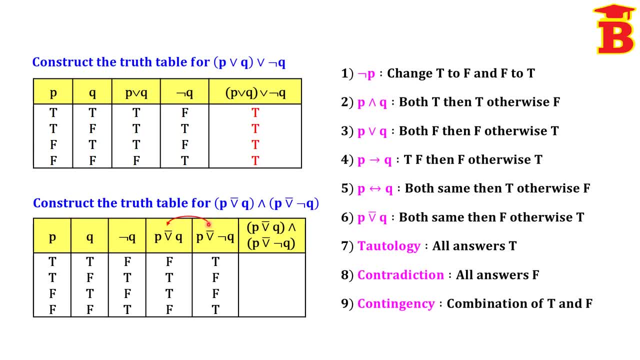 Finally, for these two we have to connect using AND And we know that AND means P and Q means both true, then true, otherwise false. So check in these two columns whether we have both true. We don't have both true, That means all the answers are false. 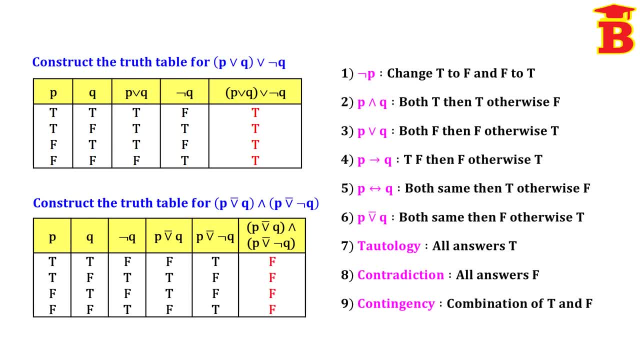 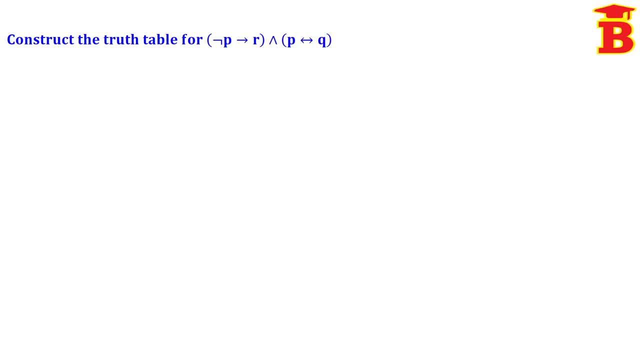 So we write all the answers false. So the final answer: FFFF. Similarly, we can construct the truth table even for three statements P Q R. See the question here. we have three statements P Q R. If we have three statements then there are eight possibilities. 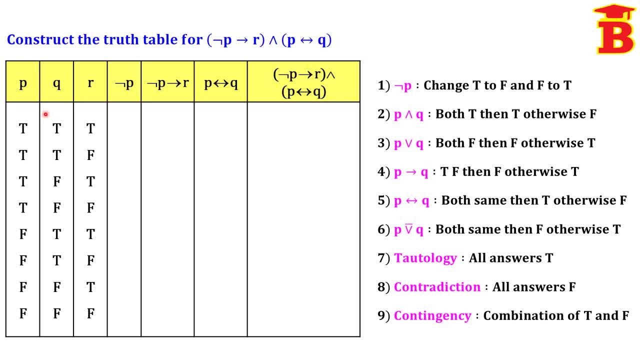 These are the eight different possibilities. This we can remember very easily. for that there is one shortcut method. First column: write four times T and then four times F. Second column: write two times T and then two times F. Two times T, two times F. 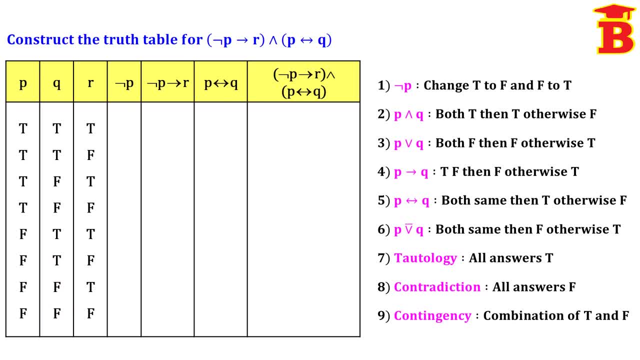 Third column. Fourth column: write single TF, TF, TF, TF. In this way we can get all the eight different possibilities. Now we have to form the table, See the question and take and write the information That is NOT P, and then first bracket NOT P, then R, and then second bracket P, if and only. 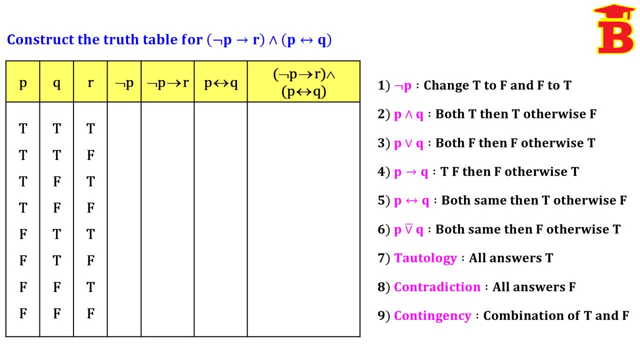 if Q And finally take the question Now. NOT P means See the statement: P change T to F, F, t, t. So first column change T to F. So first four change T to F, Next four change F to T, Next NOT P, then R. 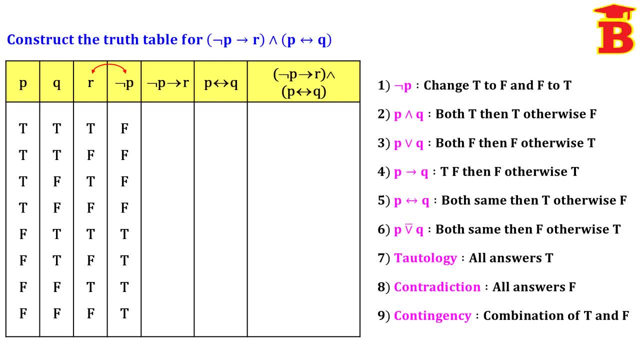 So the same thing we can write. So this is NOT P, then R, So these two we have to use conditional statement, See the conditional statement. P then Q, first true, second false. then the answer is false, otherwise true. So here not. 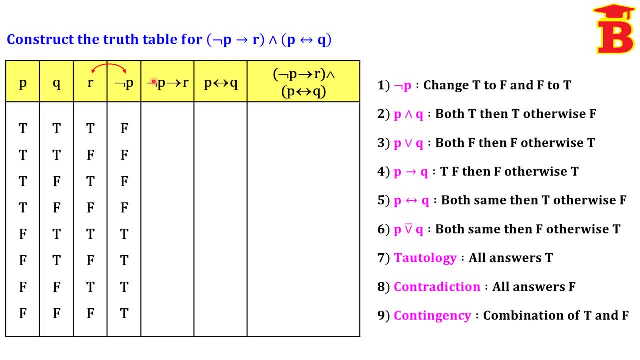 P, then R, First, not P, first true, second false. That is only these two: first true, second false. Here also this first true, second false. then the answer is false Here, first statement, not P. So first true, second false. we get the answer false, otherwise true. 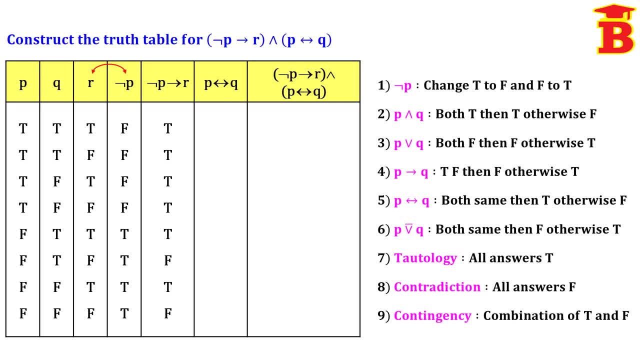 So all other answers true. Next column: P if and only if Q, P if and only if Q means both same, then true, otherwise false. So see the statements P- Q and check whether we have both same. So both same we have in first row, second row. 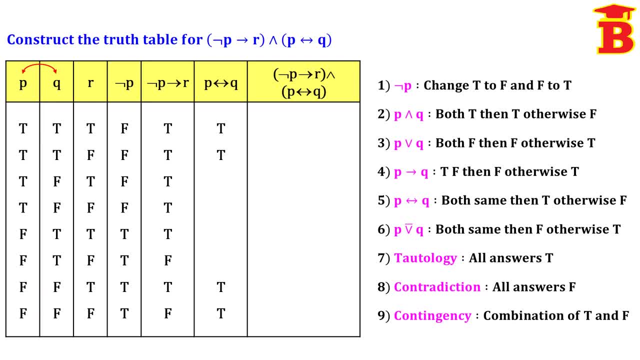 And then last two rows. For both same we write true, TT, TT, All others false. And finally these two we have to connect using AND And note that AND means both true, then answer true, otherwise false. So in these two columns check whether we have. 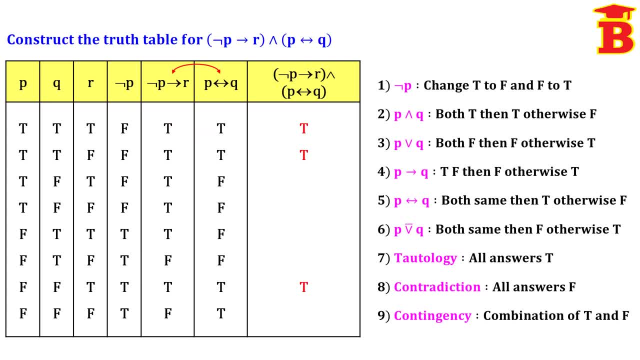 both same. So in these two columns check whether we have both true. we have both true, first, second and last before. So for that we write the answers true, Otherwise false. So all other answers false. So finally we get the answer. 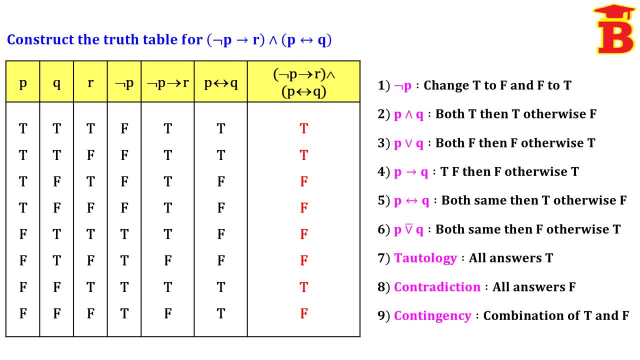 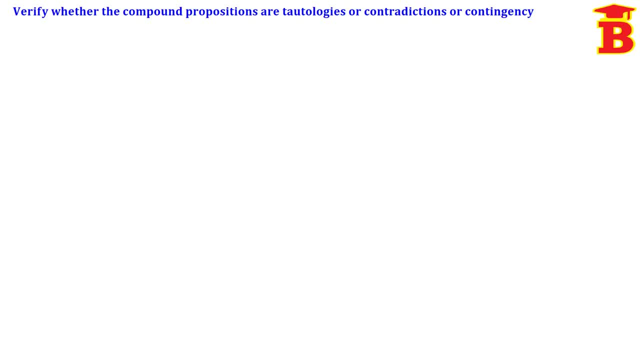 TT, FF, FF, TF. Next problem: verify whether the compound propositions are tautologies or contradictions or contingency. Here also, the statement is given. We have to draw the truth table. Based on the final answer, we can say whether it is tautology or contradiction, or 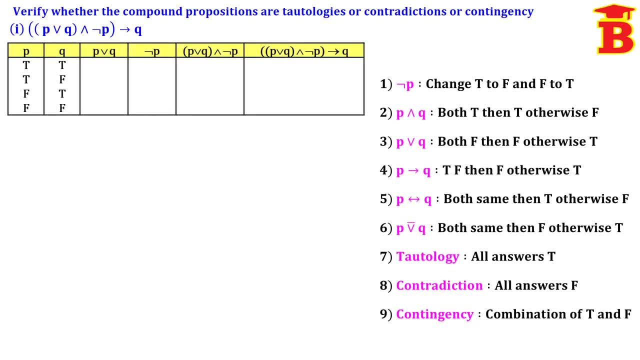 contingency P, Q. there are two statements, So four possibilities: TT, TF, FT, FF. See the question and take first P R, Q and then not P, and then this bracket P R Q and then not P. 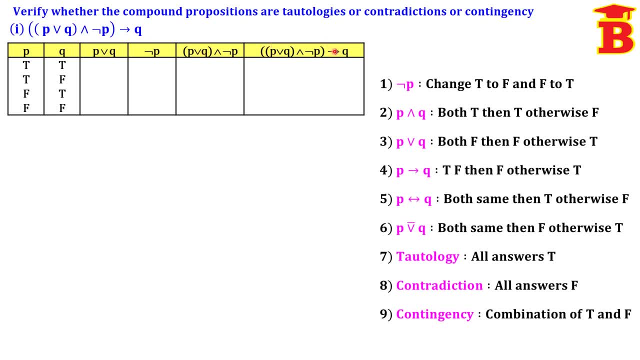 And finally take and write the question. First P, R, Q. That is both false. then false, Otherwise true. Both false. last true: That is false, Otherwise true. So all other answers true. Next, not P: See the statement. P change T to F. 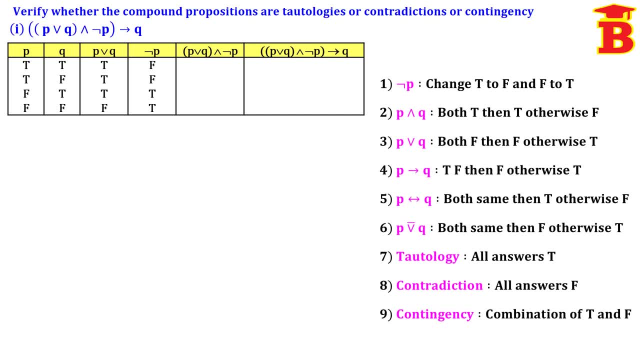 And then F to T. Now these two connect using AND. AND means both true, then true, Otherwise false. So in these two check whether we have both true. Only in the third row we have both true, So for that the answer true, Otherwise false, All other answers false. And finally, 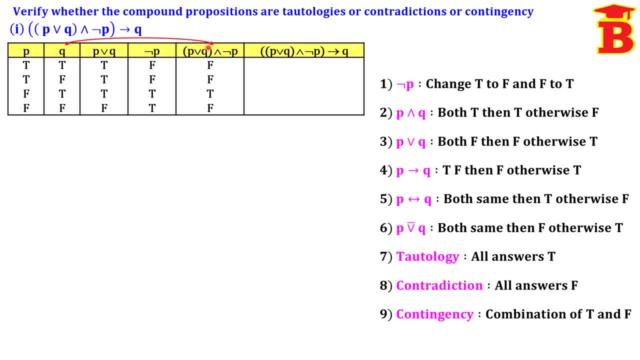 these two we have to connect using conditional, that is, single arrow mark, Single arrow mark. the condition is: first true, second false, then false, otherwise true. Here first is this bracket. so first we have to see this column: first true, second false. So here we have this first. 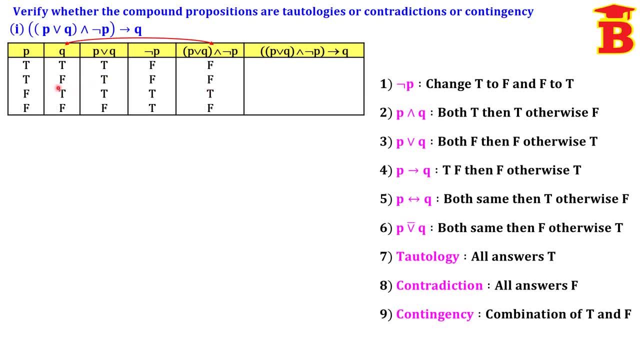 true, but we don't have false here. that means we don't have first true, second false, So we cannot get the answer false. that means all the answers true. If we get all the final answers true, then we say that it's a total. Therefore the given statement is a tautology. Similarly, second one. take the two statements. 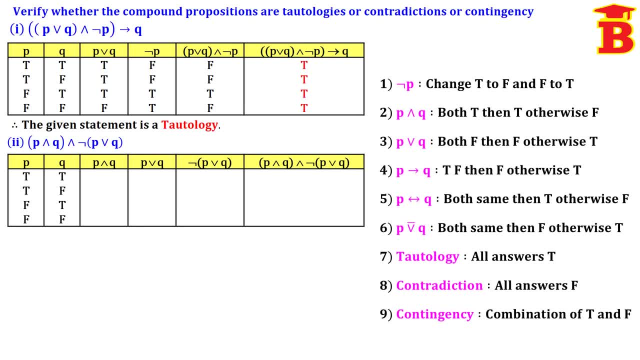 PQ. four possibilities: TT, TF, FT, FF. and form the table: first bracket: P and Q, next second bracket, PRQ and then negation of PRQ and finally take the question. First P and Q and then negation of PRQ and finally take the question. 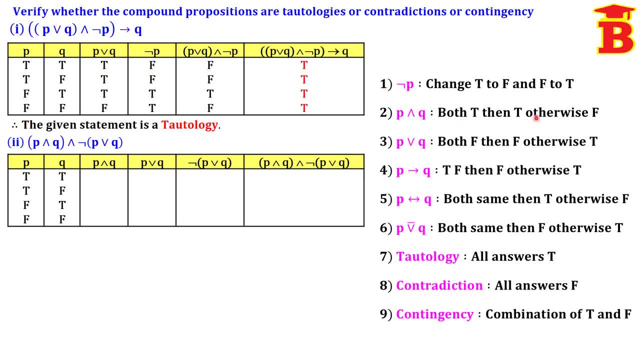 First P and Q. that means both true then true, otherwise false. So we have both true in first row. So that answer is true, otherwise false. PRQ. both false then false, So we have both false last row. So that answer is false, otherwise true. Now take negation of PRQ and then negation. 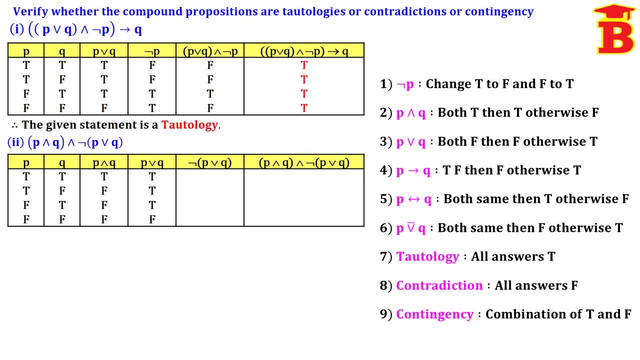 of PRQ. So negation means change T to F, F to T. So change T to F, This T also F, Next T also F and finally change F to T. Finally, for this question, take these two statements: connect using AND. AND means both true, then true, otherwise false. 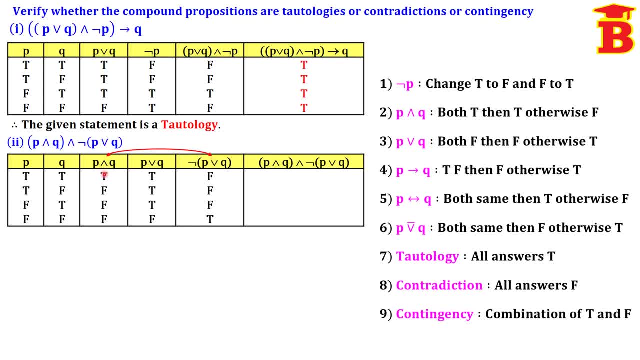 So in these two columns, check whether we have both true. We don't have both true, that means all the answers are false. So if all the answers are false, then we say that it's a contradiction. Therefore the given statement is a contradiction. Similarly, let us see the 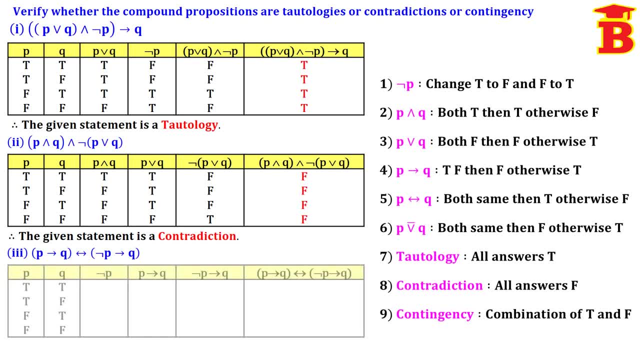 last one. Here there are two statements, p, q. So four possibilities: tt, tf, ft, ff. First take not p, and then first bracket p, then q, and then second bracket, not p, then q. Finally take the question. Here not p means we have the statement p, Just change t to f and f to t. So first t to f and then f to t. 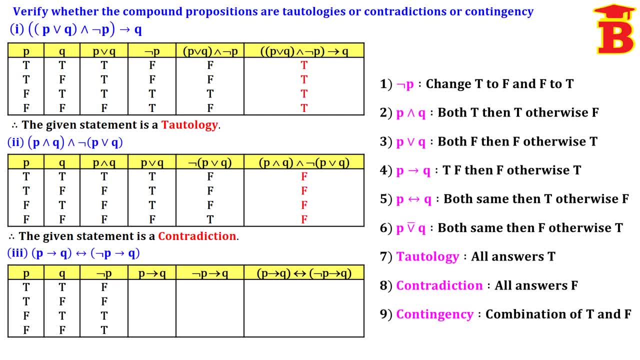 Next p, then q, P then q means first true, second false, then false, Otherwise true. So only in the second row We have first true, second false. That answer is false, Otherwise true. Next not p, then q. So this is not p. this is q, Not p. this is the first statement. 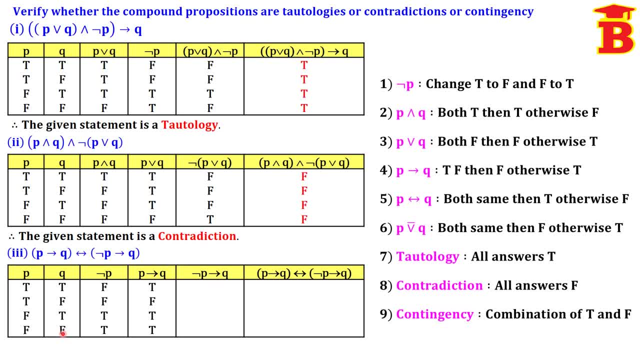 So first true, second false. Only in the last row we have that. So that is false. First true, not p true. Second false, q is false. So only this last row false, Otherwise true. All other answers true. 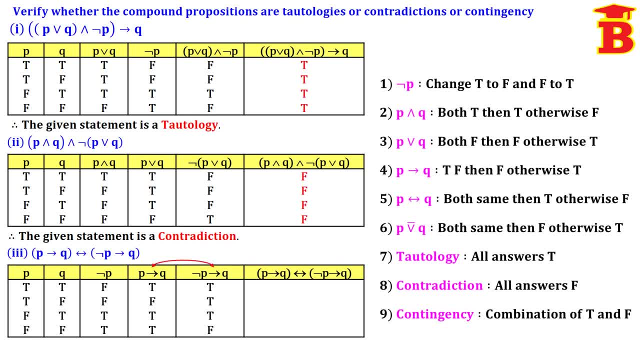 And finally these two we have to connect using biconditional. So this double arrow mark means biconditional. For that the condition is both same, Then true, Otherwise false. Both same. See these two columns. We have both same in first row and third row.